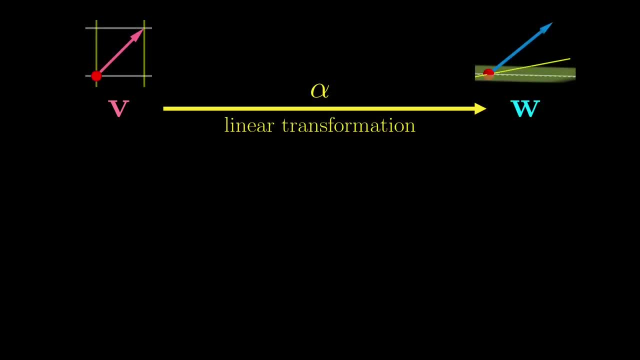 two-dimensional vector and w could be a three-dimensional one And for some reason you want to measure w. A bit of a silly analogy would be: you want to measure your own weight and the vector is u here, But you don't have a bathroom scale and you have to use your neighbors. So one way to do it would. 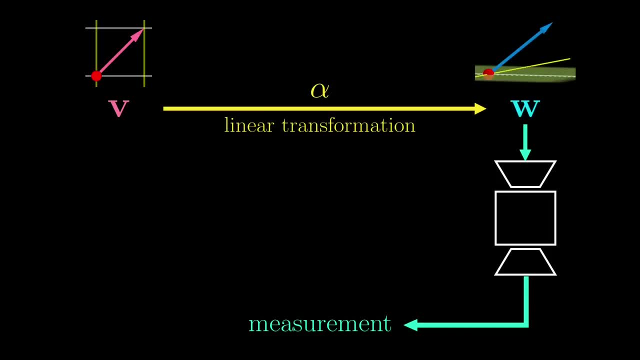 be to go to your neighbor's house then take the measurement there directly. But you could also just call the neighbor to lend you the scale so that you can take the measurements at home and get the same answer. The scale being moved from the neighbor's house to yours is the transpose of 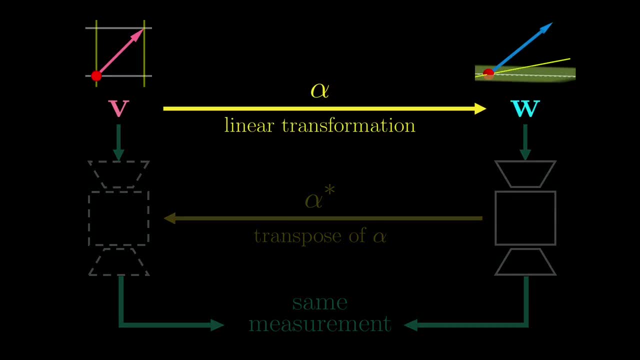 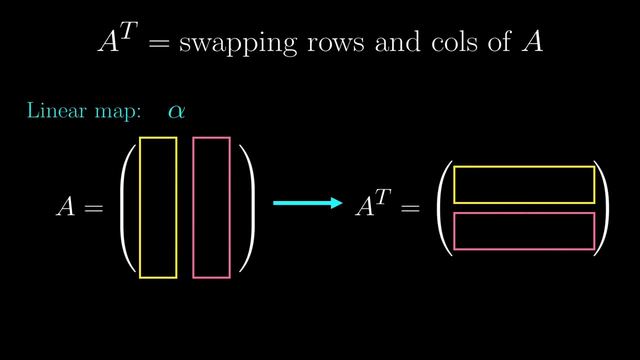 alpha. So, alpha, is u going to the neighbor's house and alpha transpose is moving the measuring device from the neighbor's to yours. But how is this related to the matrix transpose that you know? A matrix is, at its core, only a summary of a. 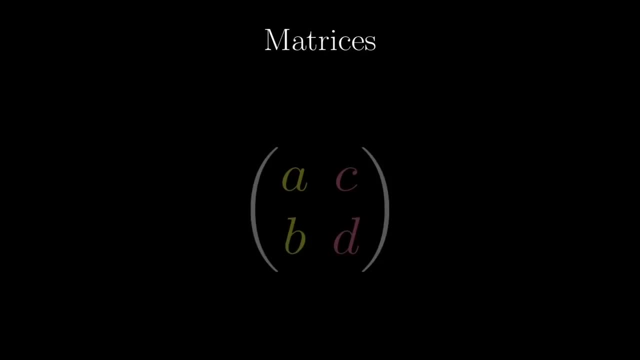 linear map. For a two-dimensional linear map, for instance, the first column tells you where the vector goes and the second column tells you where the vector goes. If we then want to know where an arbitrary vector- x, y- goes, just multiply the first column by x and the second column by x and the 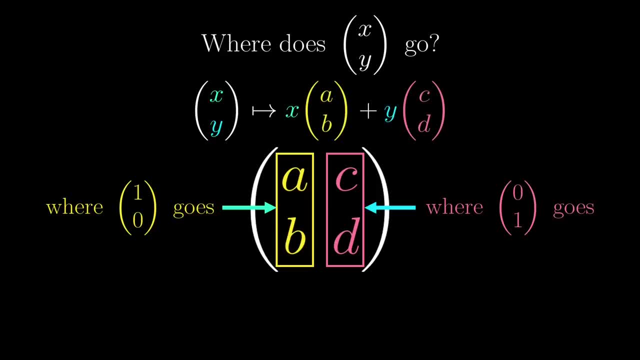 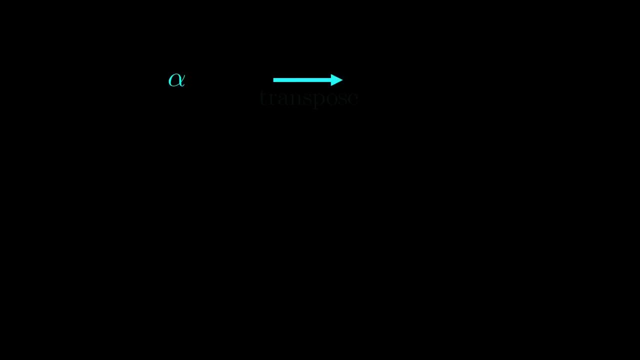 second column by x and add to y times the second column. Just knowing these four numbers is enough to determine the entire linear map. so the matrix is essentially the summary of the linear map. So you have the linear transformations alpha and its transpose and also the two matrices that are. 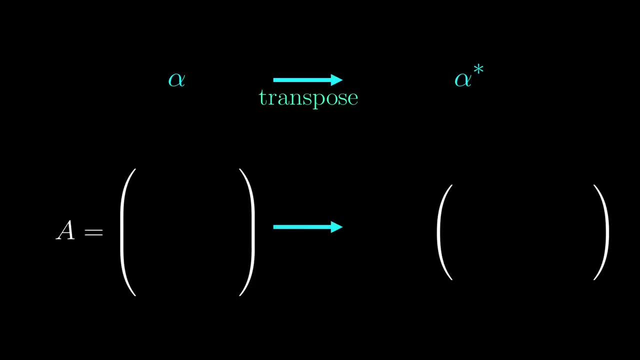 summaries of the transformations. Because the matrix on the right summarizes the transpose of alpha. it makes the matrix a sum of the transformations of x, y and its transpose. So you sense to call it A transpose. It just turns out that the summary matrices of alpha and alpha 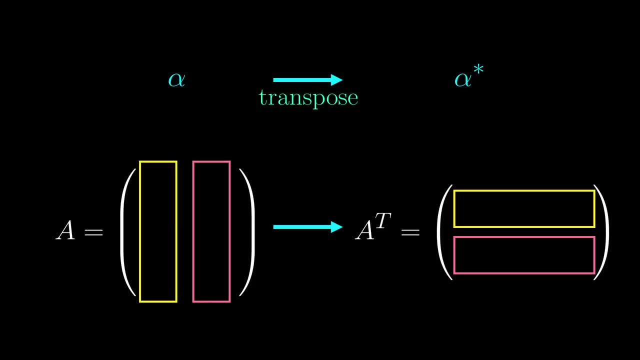 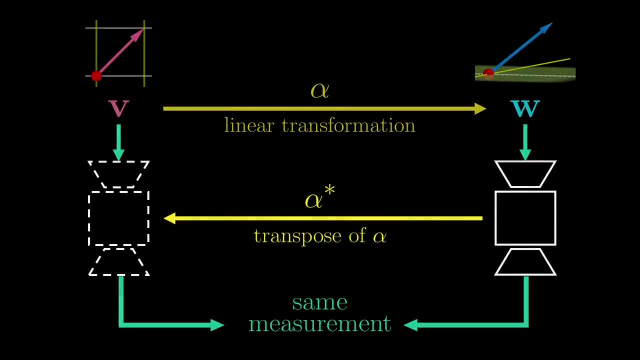 transpose can be obtained by swapping rows and columns of each other. The most important point here, though, is the big picture. A transpose is just transforming some measurement device in other spaces back to that in the original. In what remains, we will first of all: 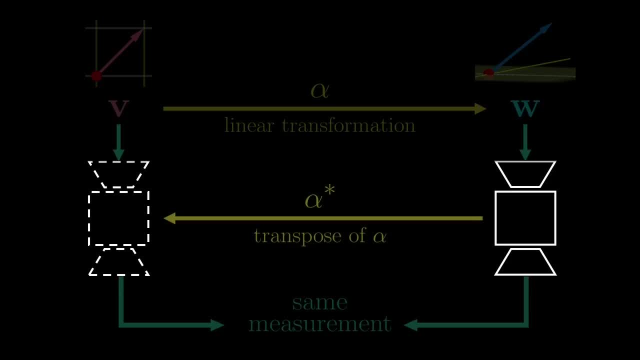 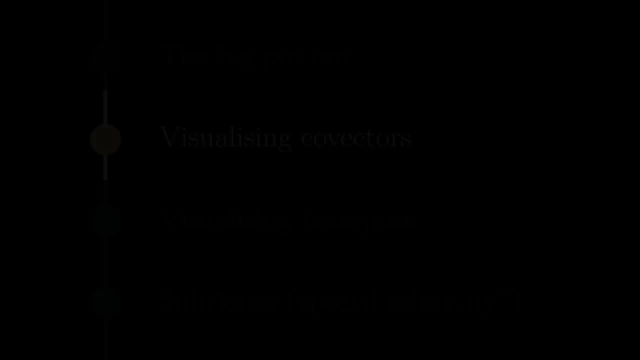 try to visualize those covectors and then the transpose Covectors are linear. so, just like our linear transformations, in the two-dimensional case it suffices to know what 1, 0, and 0, 1 are measured If the measurements are A and B. 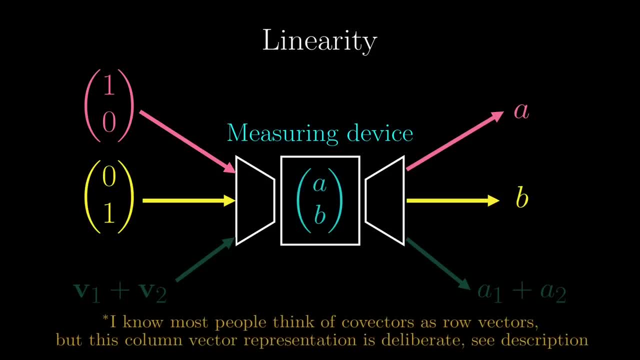 respectively. for our purpose, let's say this is an A- B covector. Now, if you take any vector x- y, you can see that the covector is a covector. If you take any vector x- y, you can see that. 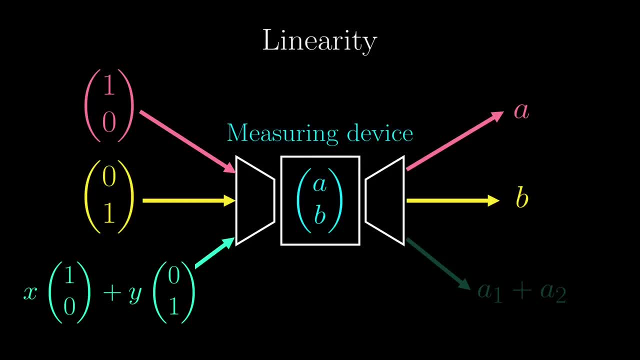 which is just x times 1, 0 plus y times 0, 1.. Just by linearity it will be measured as x times A plus y times B. So in a two-dimensional case an A- B covector measures the vector x- y to be xA. 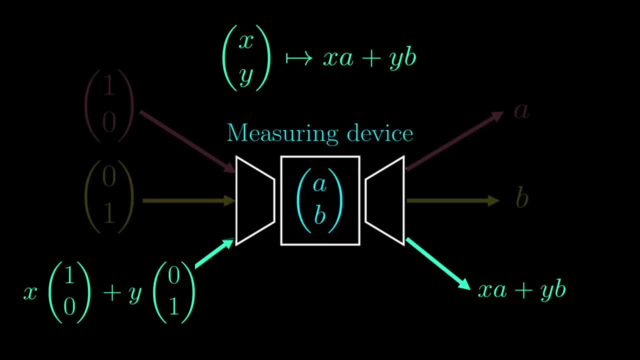 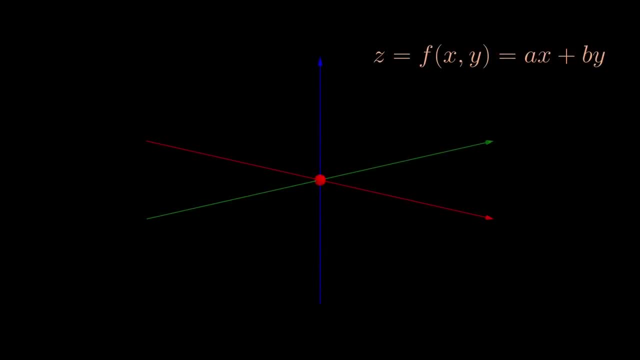 plus yB. This is just a function of two variables. A natural way to visualize this would be to plot a three-dimensional covector. If you take any vector x- y, you can see that the covector is a three-dimensional graph, with the z-coordinate being the function value at x- y, In this case. 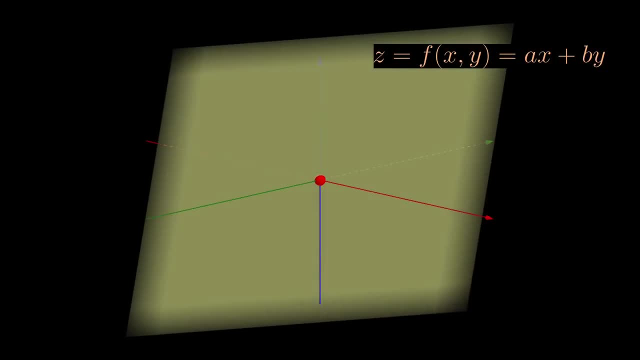 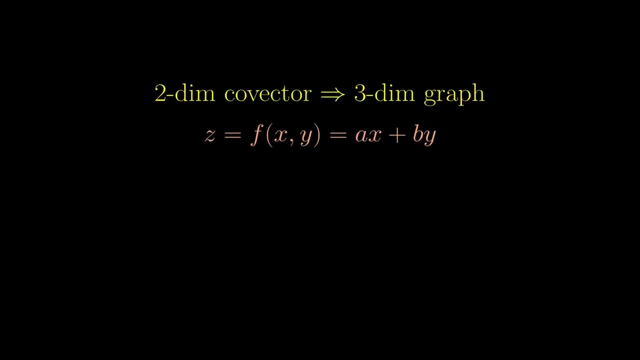 it is just a giant plane passing through the origin. However, because we might want to consider a three-dimensional covector later on, we use another, slightly roundabout way of visualizing such a function. Instead, we consider its level sets. That means you plot all the points x, y. 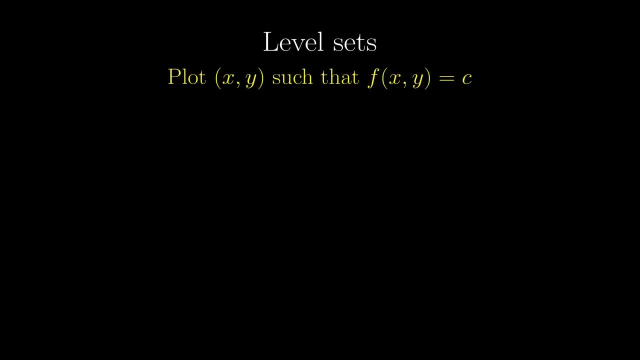 such that it gets measured as a number c. In this specific case we plot the line graph: A x plus B y equals c, where A is 2 and B is 3, so this represents a 2, 3 covector By varying c. 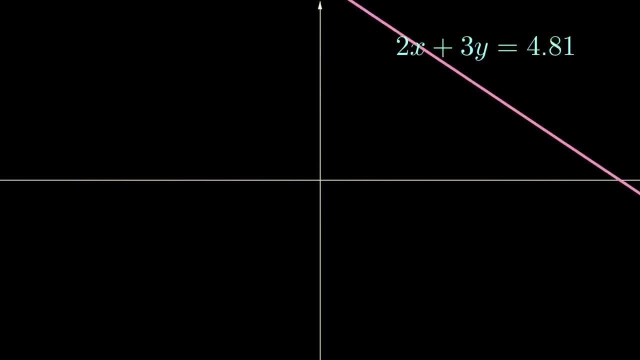 we get a glimpse of how this function behaves In this case. it just moves up and down. We label this line to be 1, because that's all the points that will be measured to be 1.. And we only draw a line graph for, say, integer values of c. so we have parallel lines at regular. 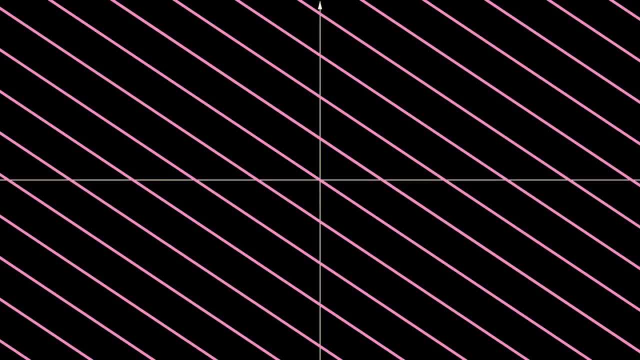 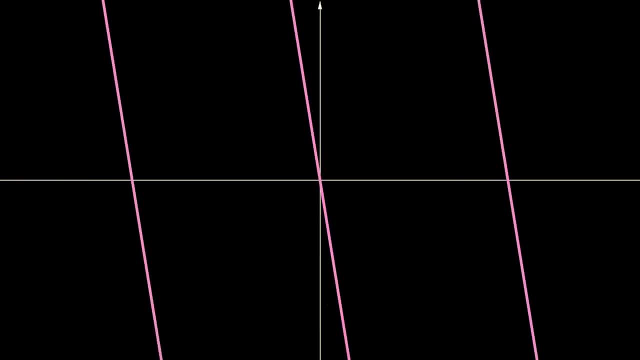 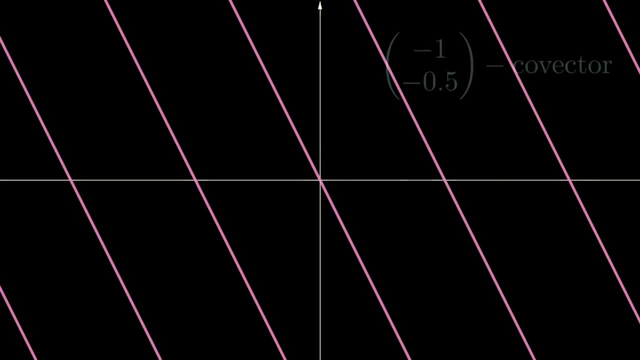 intervals. Of course, this is just one covector. Different covectors will have different sets of parallel lines with different directions and densities. But now the question is: given a particular set of parallel lines, can we quickly spot which covector this is? 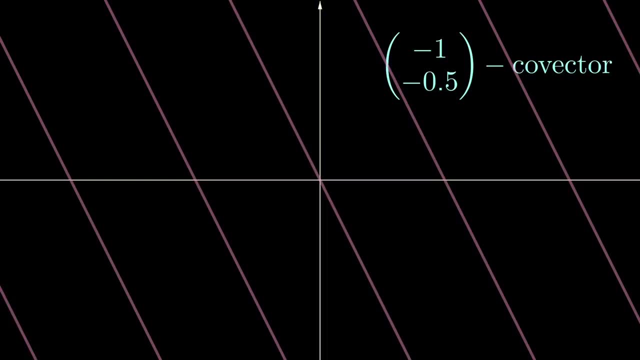 In this case it is the negative 1, negative 0.5 covector. So let's compare with the negative 1, negative 0.5 vector and see what happens. The corresponding vector is perpendicular to all the lines. So okay, given these parallel, 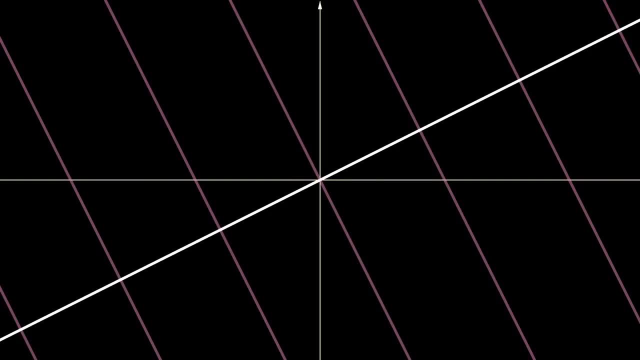 lines. all we know is that the corresponding vector lies on this perpendicular line, But why is this exact vector then? If we scale this vector, we notice that the longer the vector, the more the vector will be perpendicular to the line. If we scale this vector, we notice that the 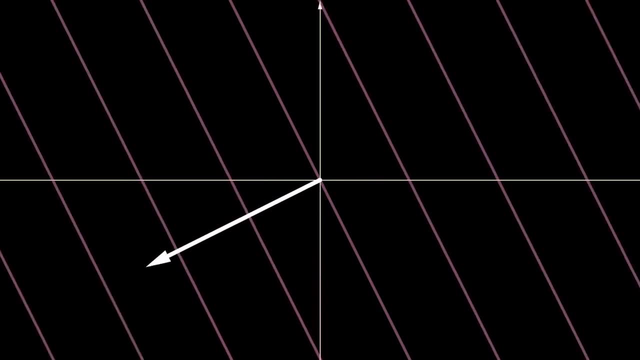 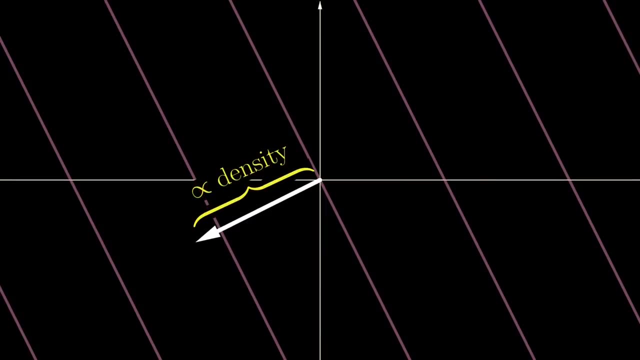 right line is possessing both sibling lines. So I'm going to put the radar vector at 50, and let me know how this Main IC will react. So I'm going to put the radar vector at 180.. And now I'm going to add this linear matrix. 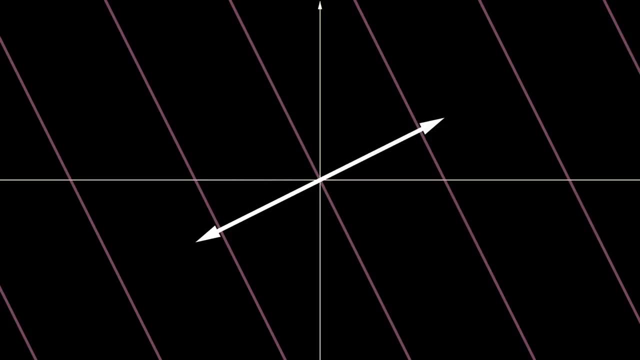 So I'm going to compute this linear matrix by using Bayesian coefficients, then by adding the delay value, and I'll show you how to do it next. know the length, but these two vectors have the same length. How do you determine which one? 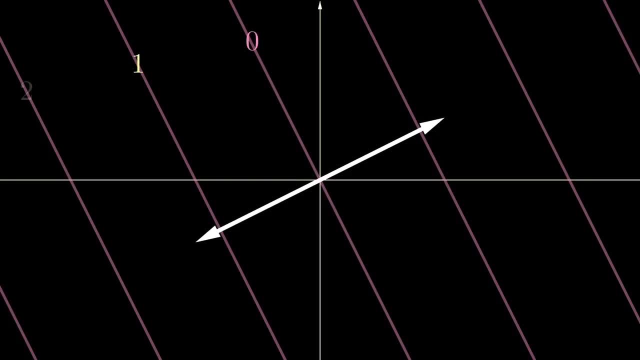 It's actually impossible to tell unless you label back those lines. This line, for example, was labeled 2, because they are all the points where the covector would measure them to be 2.. With these labels, we can tell these two vectors apart. The corresponding vector points towards. 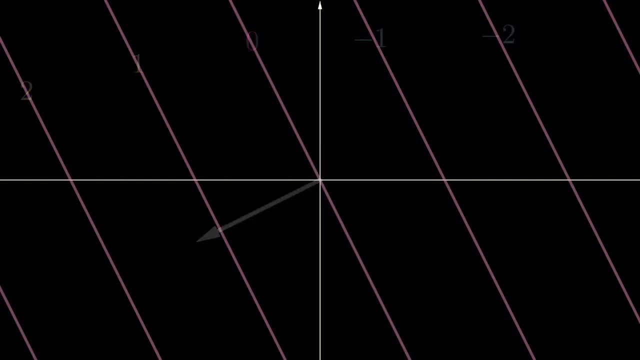 positive labels. So here is a summary of how you know which covector you have, just by looking at these lines. First off, you know the corresponding vector is perpendicular to the lines, so the vector must be on this white line. You take a look at the gap size. 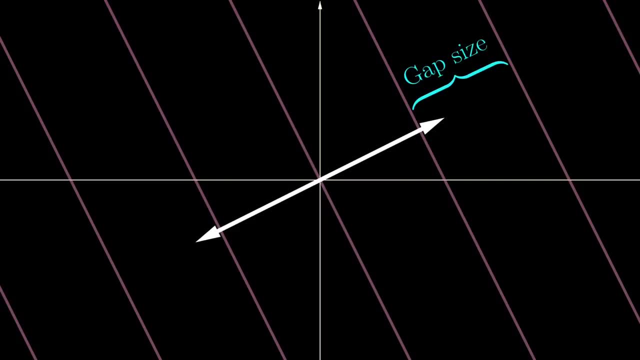 between the lines. then you know it's one of these two vectors whose length is 1 over the gap size. Then you take a look at the hidden labels of the lines and you use these two vectors to determine the covector. Choose the one pointing towards the positive labels. 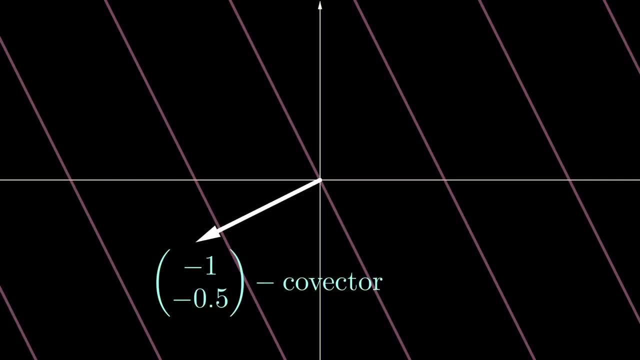 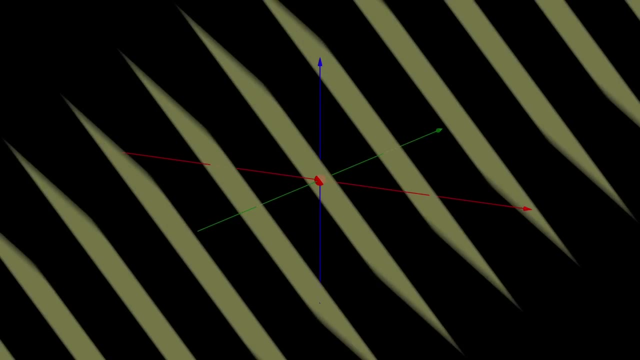 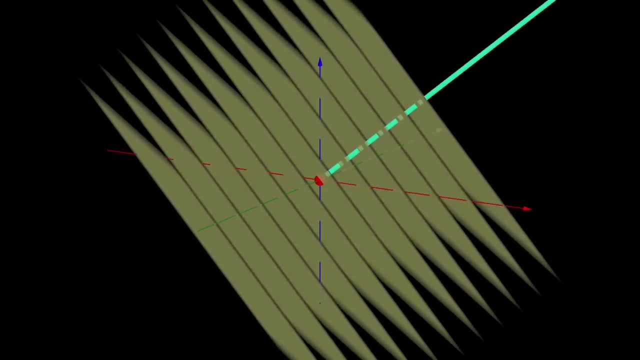 Finally, you read off the coordinates of the corresponding vector. So we have visualized two-dimensional covectors using parallel lines. Three-dimensional covectors are similar, except we have parallel planes instead. The corresponding vector would still be perpendicular to the planes. the length of the vector would still be the density or 1 over the gap. 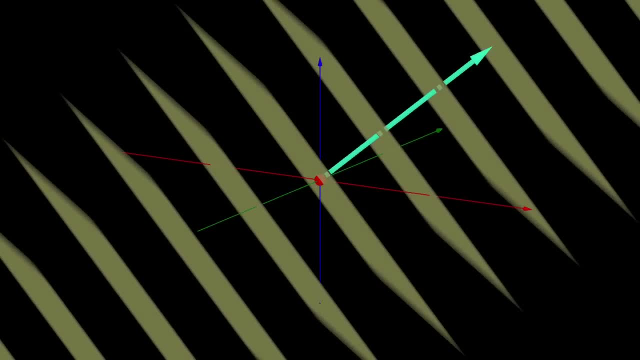 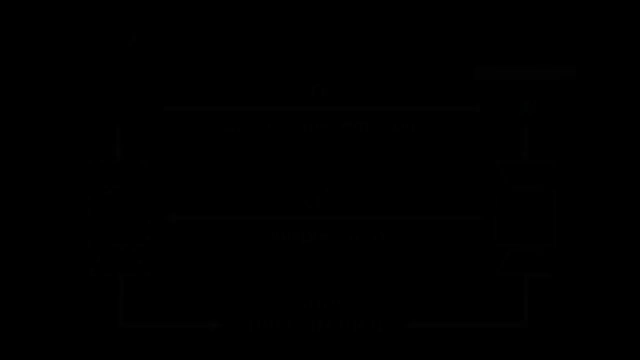 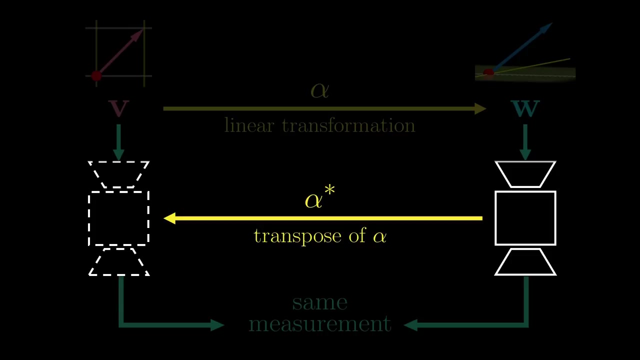 size of these parallel planes and the vector still points towards the positive labels. Now that we have visualized covectors, we are ready for the transpose, As we have seen in the big picture of transpose alpha, transpose transforms a measuring device, a covector, in the other space, back to the original space. So we transform a covector. 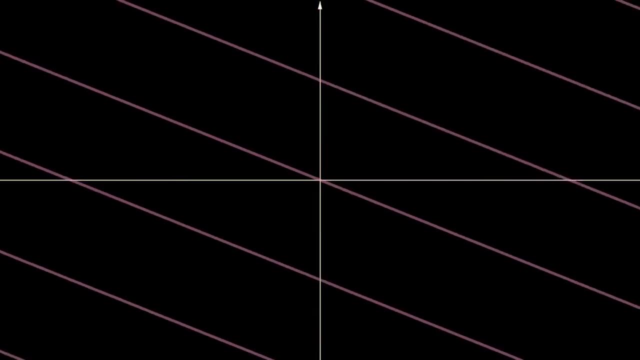 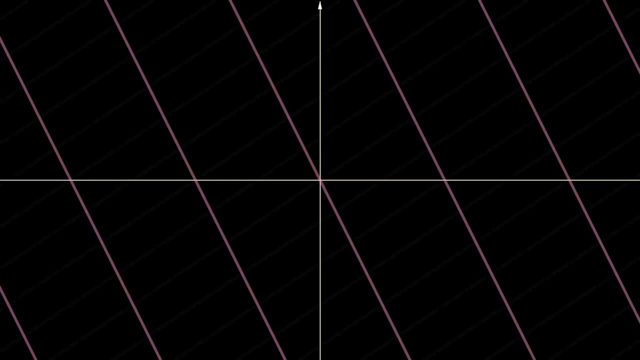 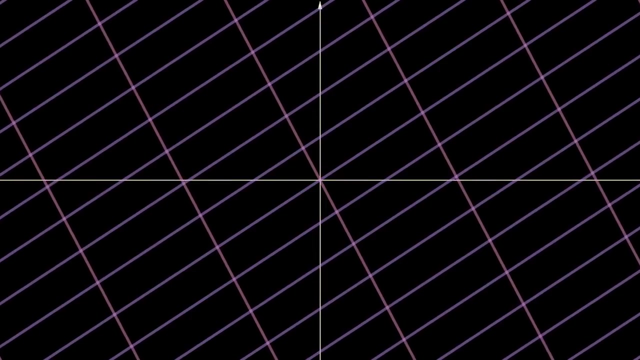 to another covector with the transpose. The trouble is that one covector already occupies quite a lot of space. Two covectors appearing together is already the maximum, So we can only visualize the transformation of two covectors at once. Which two covectors should we choose? 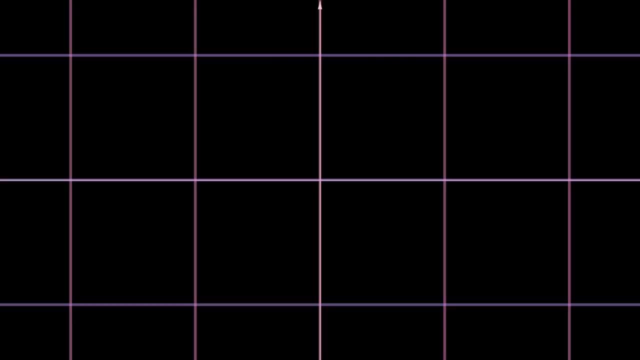 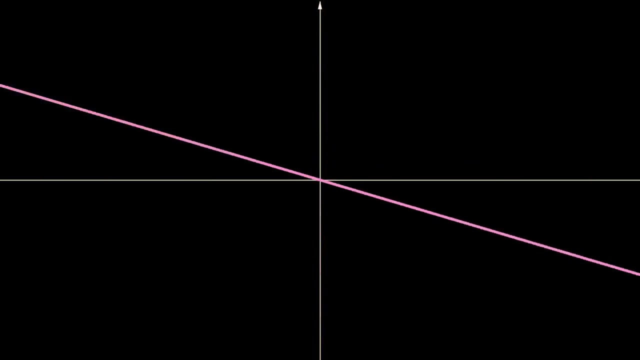 Just like normal linear transformations, the two representatives are the one-zero covector as well as the zero-one covector. Like a normal vector transformation, we observe where the one-zero covector goes. Whichever covector it becomes would be our first column of the transpose matrix. 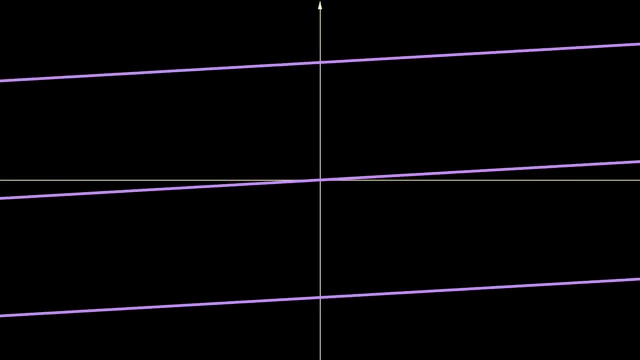 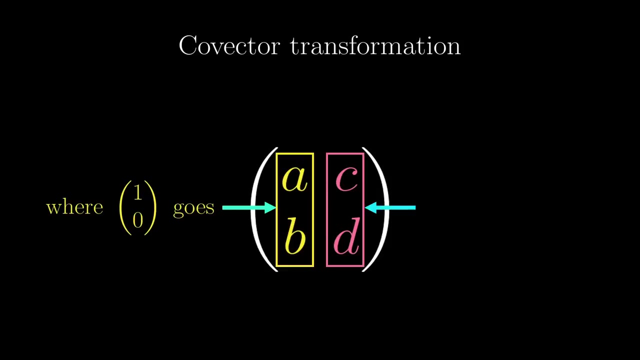 Similarly we observe the transformation of the zero-one covector. So for a covector transformation we can similarly write down a matrix representation. The first column tells you where the one-zero covector goes, and the second column tells you where the zero-one covector goes In what follows? 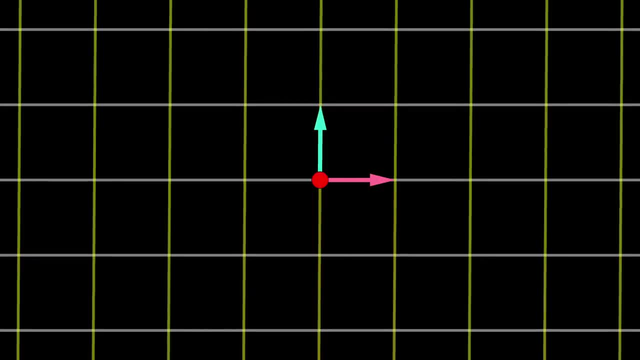 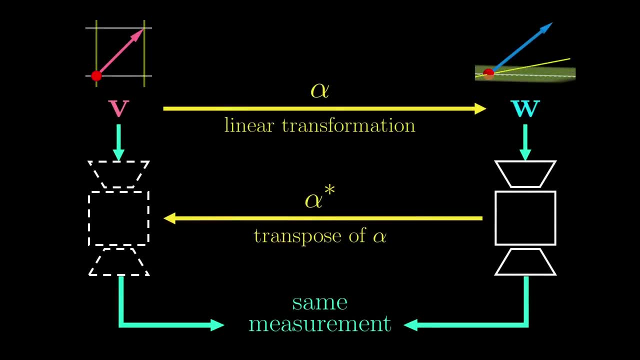 we will use the right shear as an example. What should the transpose of a right shear look like? We will need to go back to this big picture. In this specific case, alpha is a right shear and we now just have a 2D to 2D transformation. Now this one-zero covector measures the sheared. 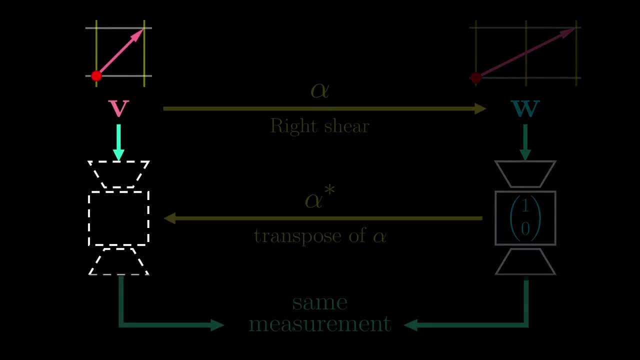 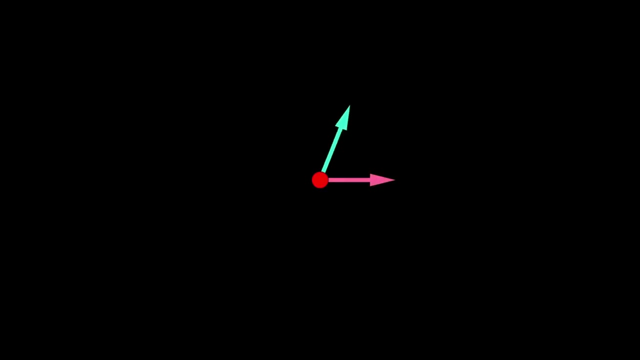 vector, And the job of the transpose is to find out which covector could we use to directly measure the original vector, such that we get the same measurement at the end. Now go back to the visuals. A right shear would transform the basis vectors as such. 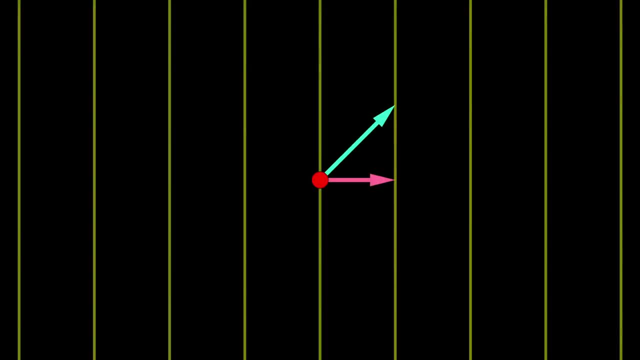 Next we see how the one-zero covector measures our sheared vectors. In this case, the measurements are both one, But rather than thinking about their exact measurements, just notice the tips all lie on this line. Remember that each line represents the tips of those vectors whose measurements are. 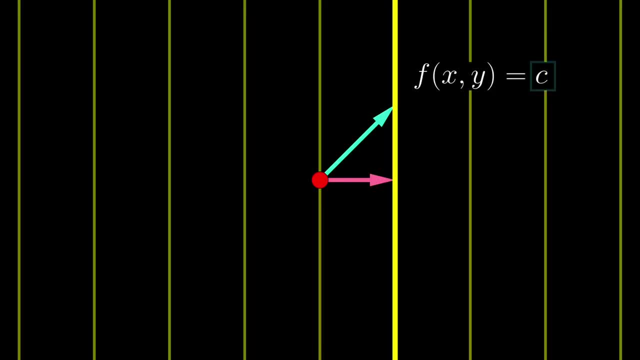 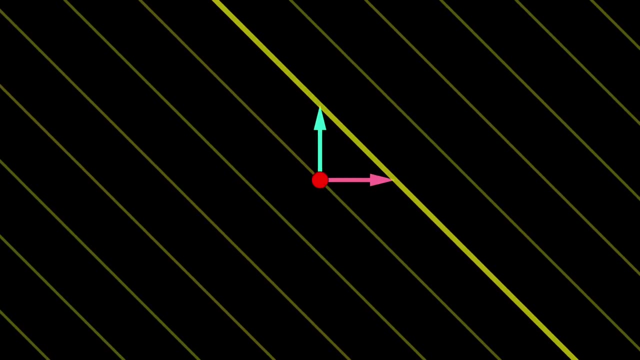 the same fixed constant c. So in this visualisation, which line the tip of the vectors are on tells you the measurement of the vectors. This is why the transpose does this First off, the basis vectors have gone back to their original place And the tips of both vectors still lie on. 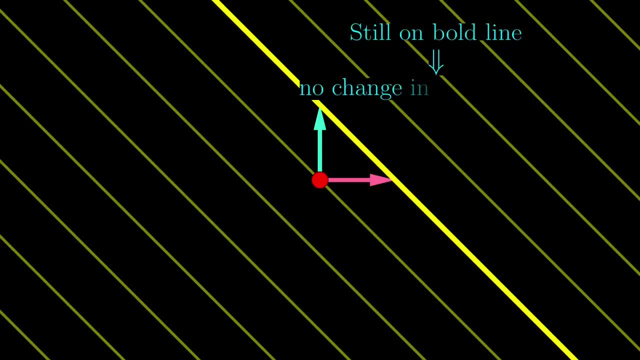 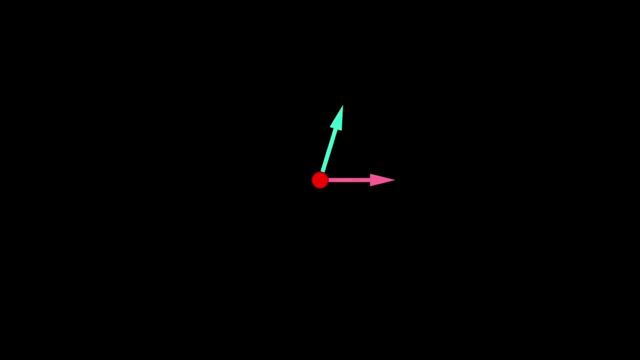 the bold line, which means that you get the same measurements as before. This is exactly what a transpose should do. Anyway, let's see what the transpose does to the zero-one covector. instead. Again, we do the right shear to the basis vectors, then use the zero-one covector to 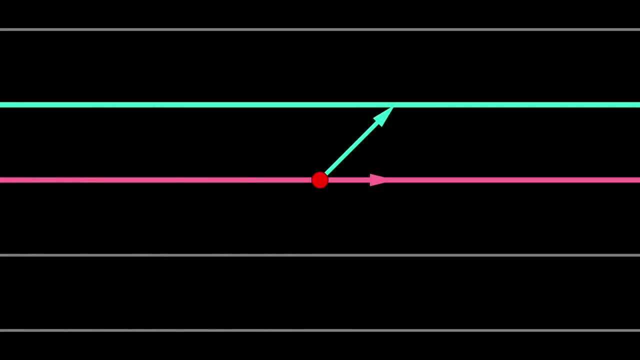 measure them. This time their measurements are different. I use the bold pink line to indicate the measurement of the pink vector and the bold green line to indicate the measurement of the green vector. For the transpose, we want to bring back the basis vectors and retain the measurements. 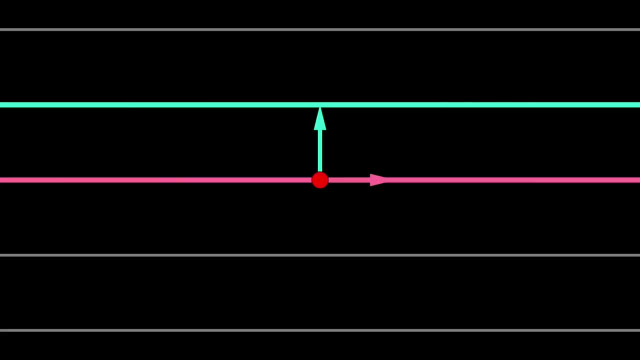 This time we don't need to do anything to the covector because the tip of the pink vector still lies on the pink line and the tip of the green vector still lies on the green line. Their measurements are not changed when the vectors go back to the original place. 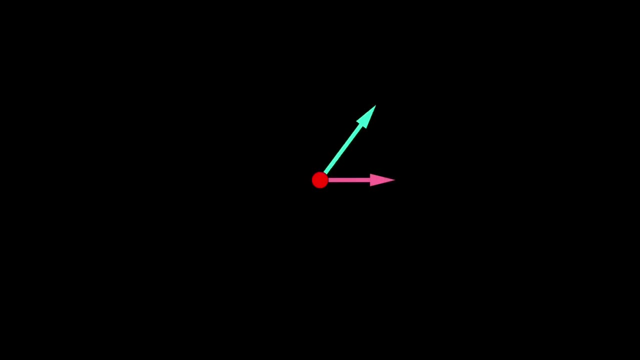 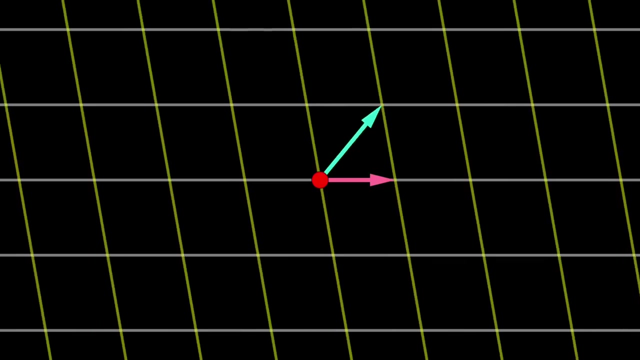 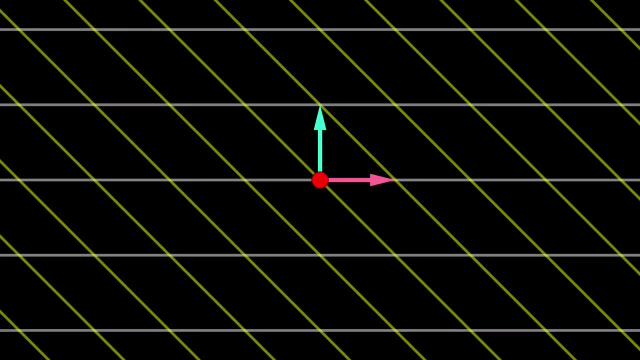 So altogether, this is the situation. after you have done the right shear to your basis vectors, The transpose wants the basis vectors to go back to the original place while retaining the measurements, So it essentially does a left shear to the whole picture. Wait, originally we have a right shear and somehow the transpose is a left shear. 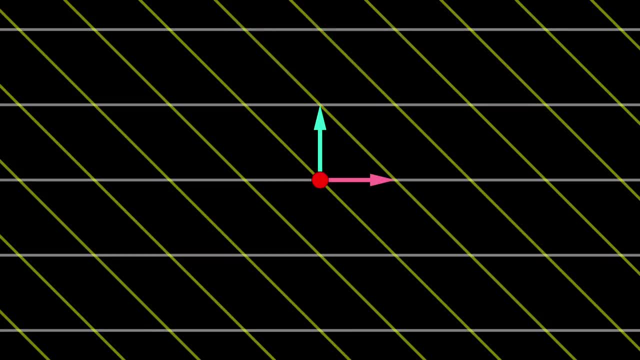 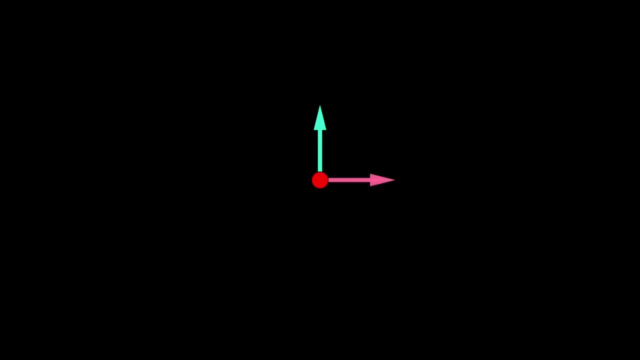 While it looks like a left shear, the gridlines are actually made up of two separate different covectors. The original right shear has the matrix 1 1 0, 1, because the 1: 0 vector stays put and it is still 1: 0 after the shear. 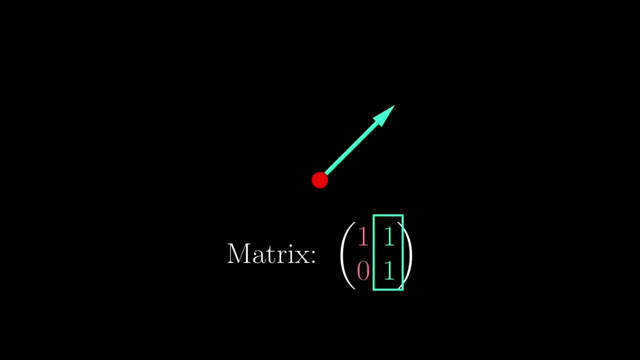 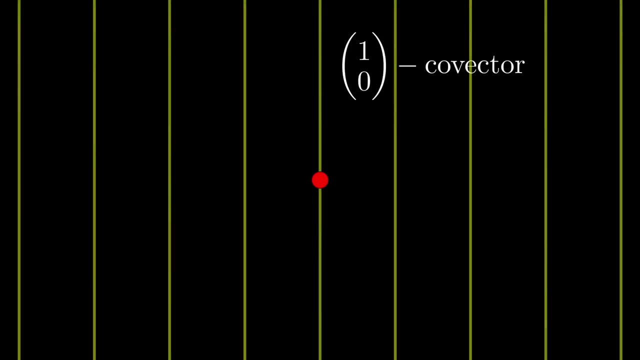 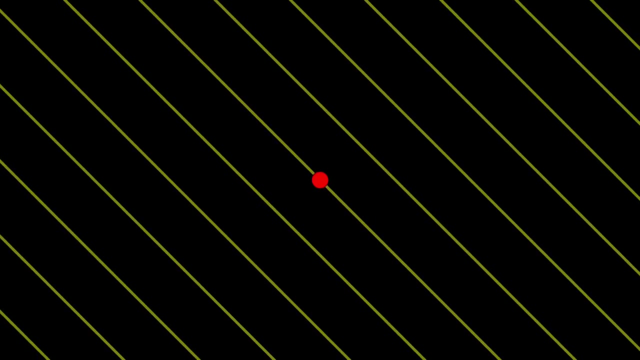 But the 0: 1 vector has sheared to the 1: 1 vector. Compare this with the transpose. This is the 1: 0 covector. The so-called left shear transforms such a covector to this one. Which covector is this? 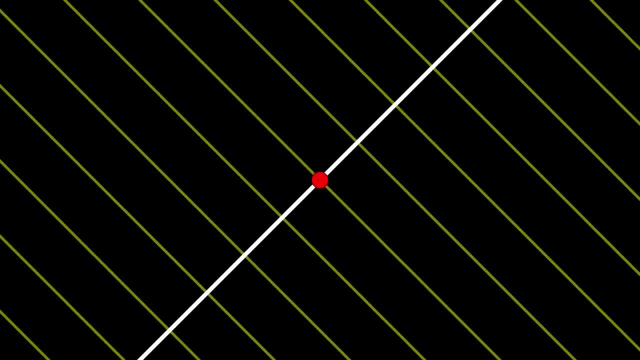 We know the corresponding vector lies on this perpendicular line. then we need to figure out the gap size. With the help of this vector telling us how long one unit is, the gap size can be calculated to be 1 over square root of 2.. So, because the length of the 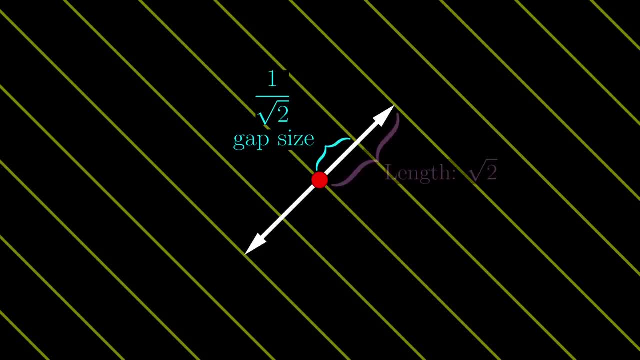 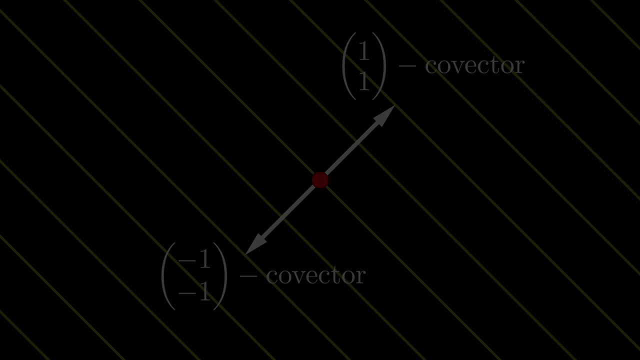 corresponding vector is 1 over the gap size. the length is now square root of 2.. This leaves us with two choices: either a 1: 1 or a negative 1. negative 1 covector, Because originally this bold line is measured positively by this 1: 0 covector. 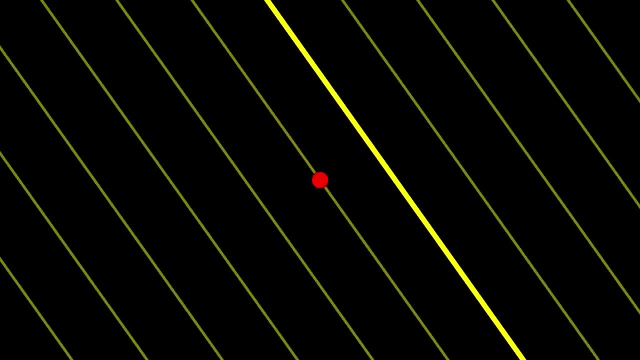 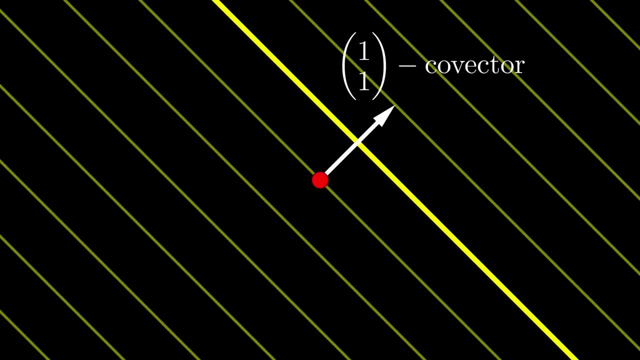 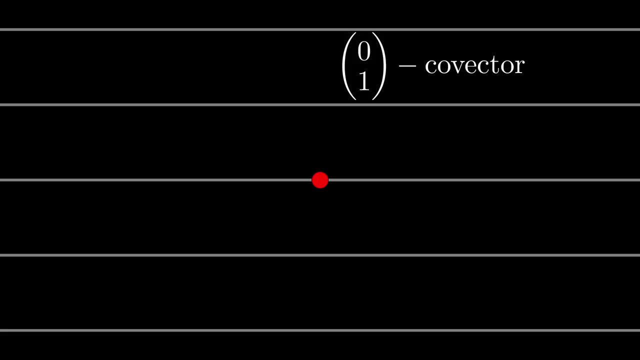 after the transformation. this bold line indicates the positive direction, and so it must be the 1: 1 covector. On the other hand, the 0: 1 covector is unaffected by the left shear, so it stays a 0: 1 covector. So this so-called left shear should be represented by 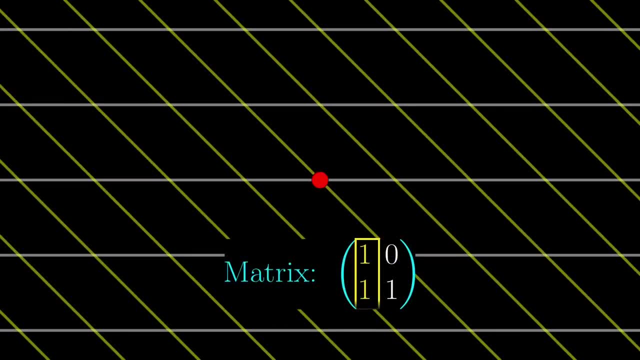 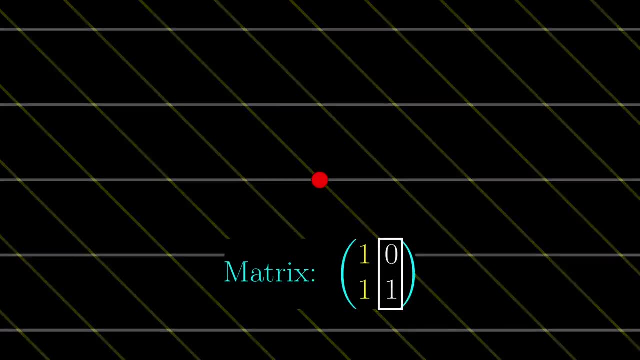 this matrix because the first column tells us that the 1: 0 covector has transformed to this 1: 1 covector and the 0: 1 covector has just stayed put, still being the 0: 1 covector. 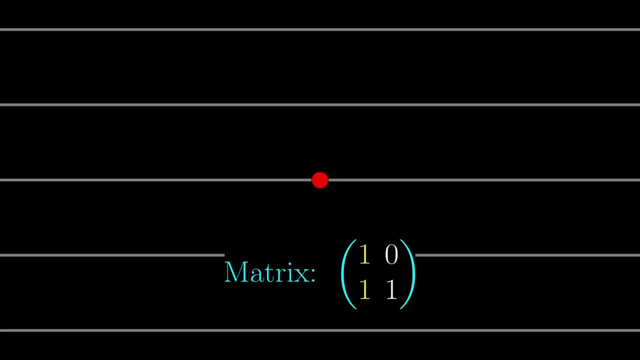 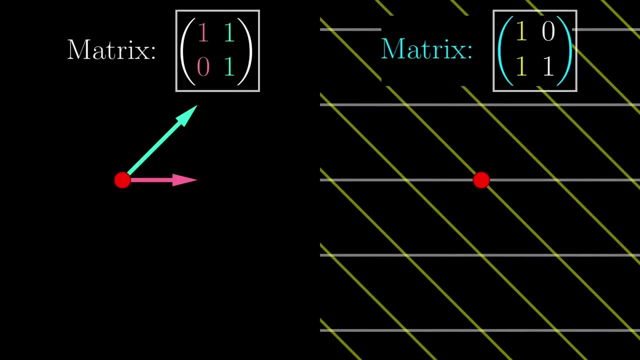 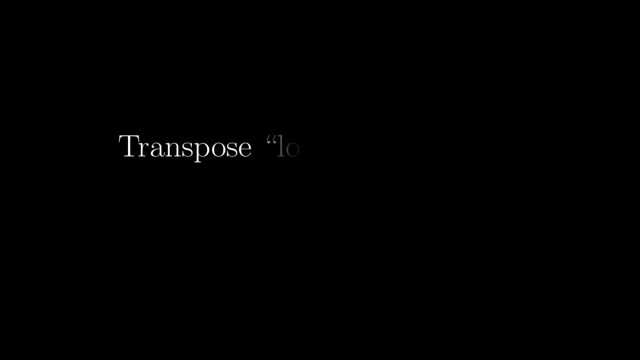 Now compare this matrix of this so-called left shear with the original right shear. You can see that the matrices are indeed just swapping rows and columns of each other. We will have more examples later on, but this hopefully convinces you that the transpose 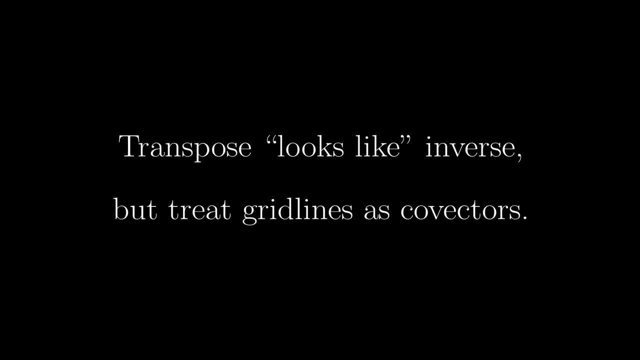 looks like inverse, but you have to treat those grid lines as covectors instead. The first of the two other examples I would give would be a diagonal matrix, such as the one with entries on the diagonal. The first column just tells us to enlarge the 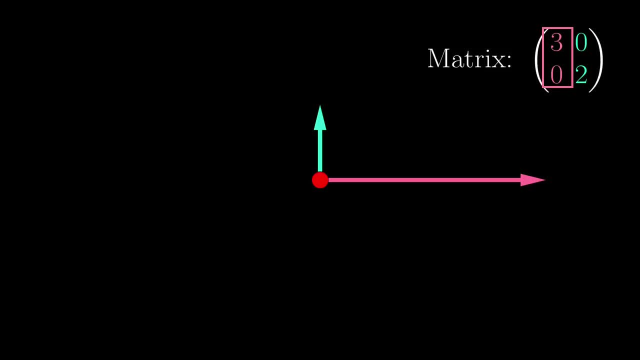 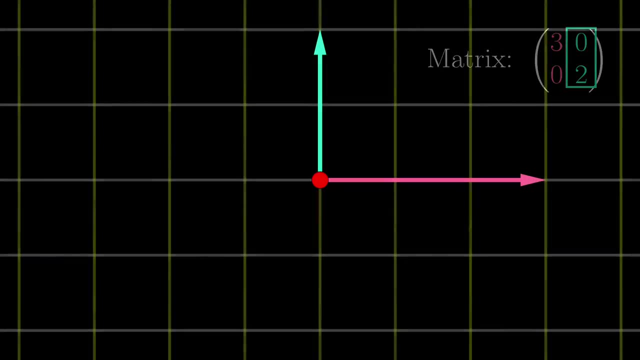 pink vector by a factor of 3, and the second column tells us to enlarge the green vector by a factor of 2.. As before, we bring on the covectors and do the inverse transformation to get the basis vectors to where it started. 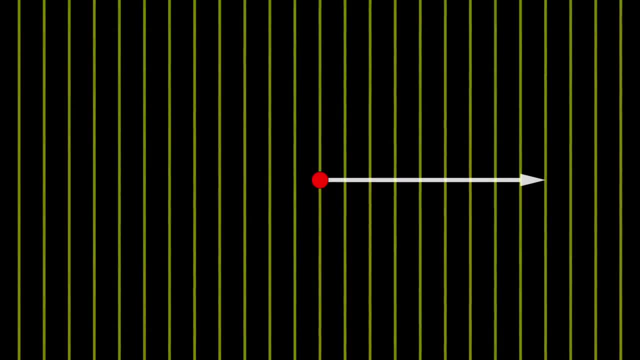 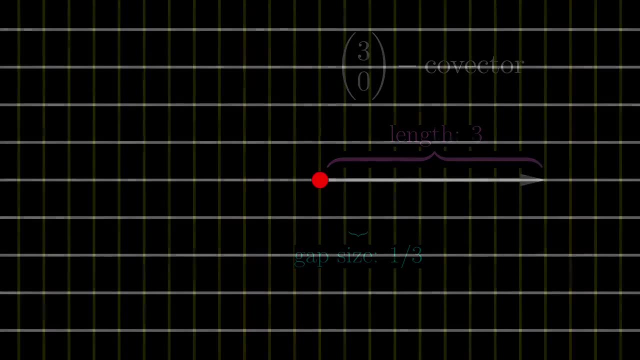 But when viewed as covectors, this is actually a 3: 0 covector, Because the gap size has now reduced to 1, 3rd to the original size. the length of the corresponding vector is actually 3.. Exactly the same story for the other covector, except the gap size is just halved. so the length 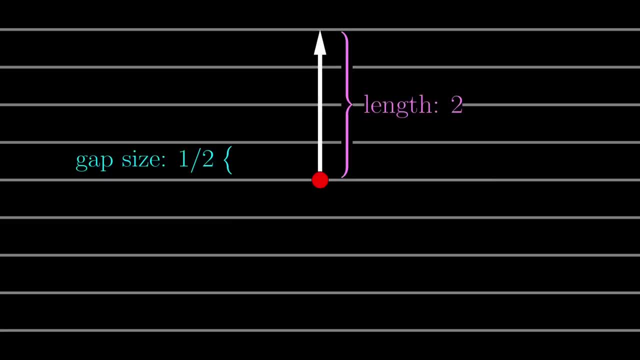 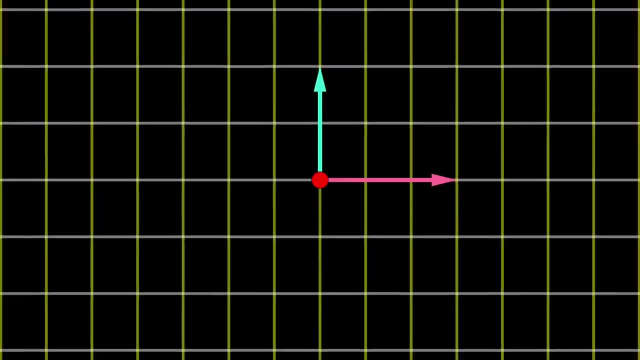 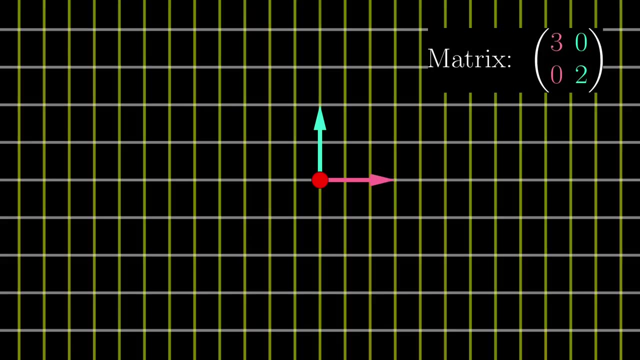 of the corresponding vector is 2.. So we end up with a 0, 2 covector. This is why this transformation is still represented by the same matrix, because we view those grid lines as covectors And indeed, if you do the swapping rows and columns thing, you still get the same matrix. 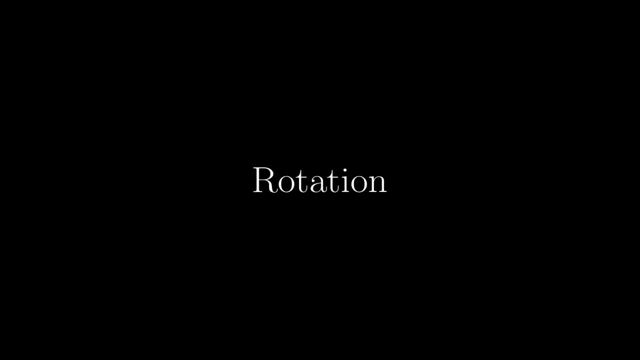 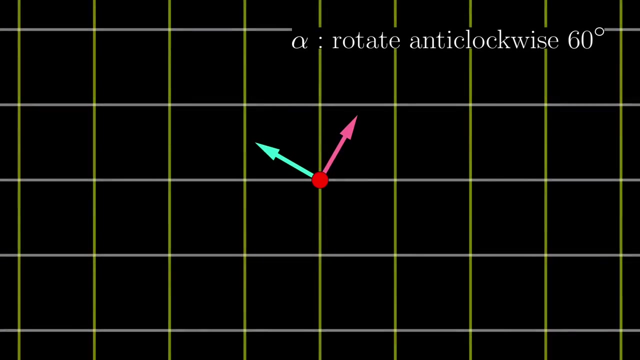 Another example would be a rotation. Again, we start off with these basis vectors and let's say we rotate anticlockwise by 60 degrees. This is our linear transformation. As usual, we bring on the covector grid and do the inverse transformation to get the basis vectors to. 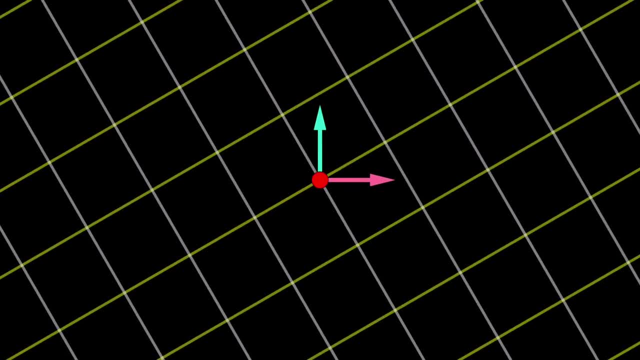 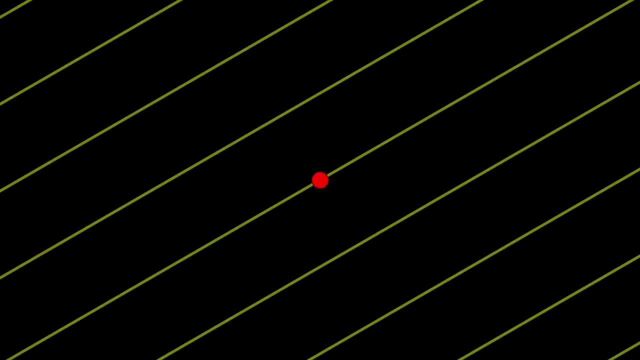 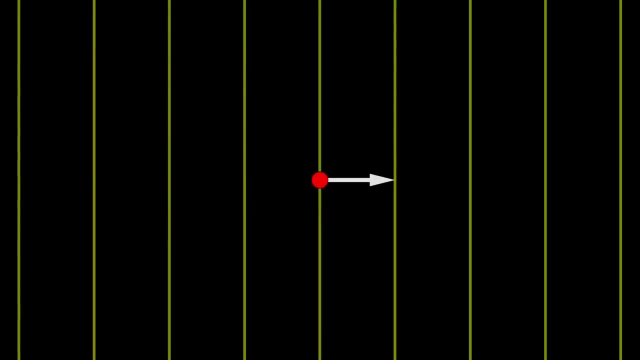 where it started. This time we rotate clockwise by 60 degrees. What is this covector then? Well, it is from rotating this original covector clockwise by 60 degrees and this is the original corresponding vector During the rotation. the corresponding vector. 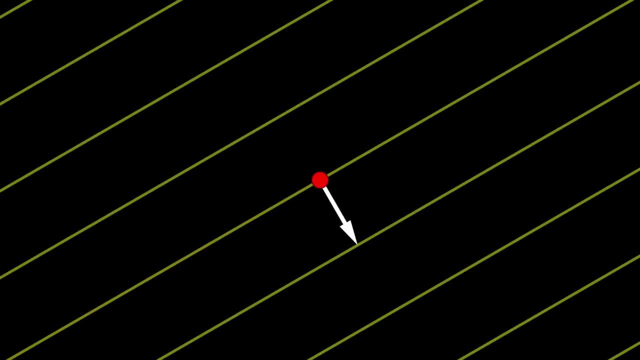 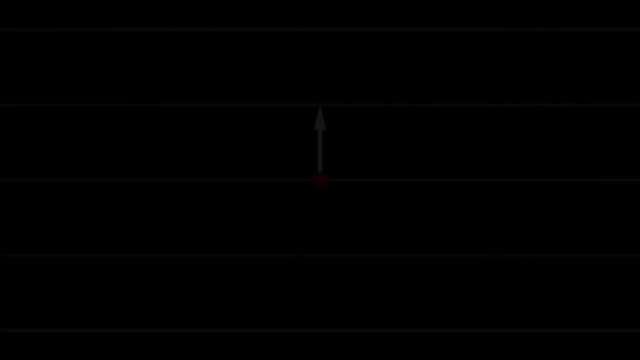 rotates the same way, clockwise 60 degrees. This is because the gap size hasn't changed, just by rotation, so we don't need to change the length of the corresponding vector. The same story for the other covector. So in this case the transpose doesn't just look like inverse. 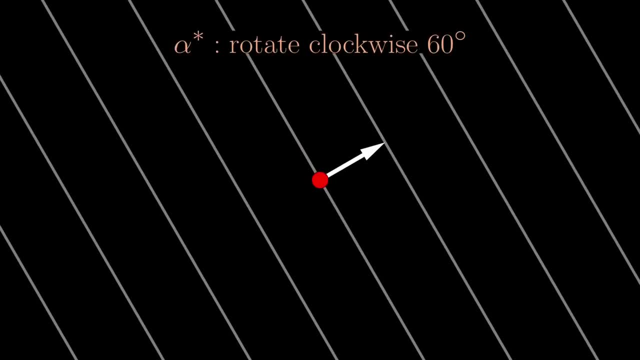 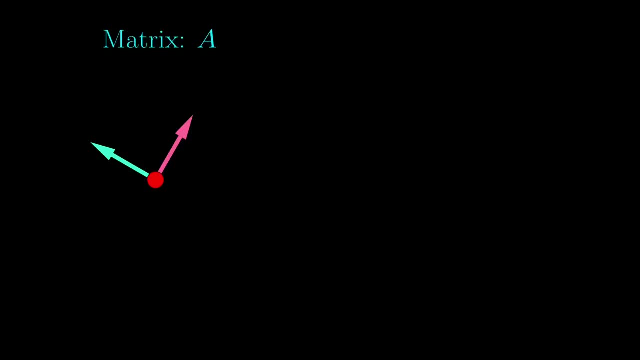 it is the inverse and it is the covector. So in this case the transpose doesn't just look like inverse, it is the inverse when acting on the corresponding vector. That means, if I write down the matrix corresponding to anticlockwise 60 degree rotation and the corresponding transpose, in this case, 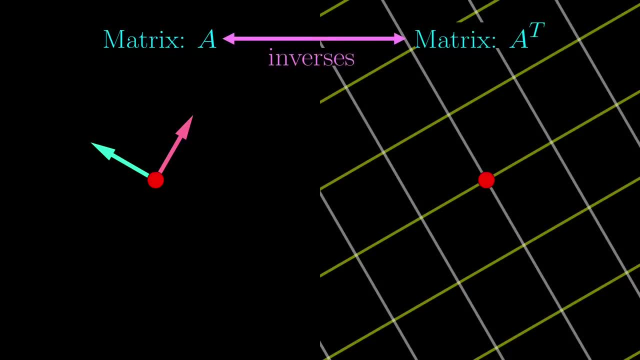 are inverses of each other. In other words, for rotation A transpose equals A inverse. In general, matrices satisfying this are called orthogonal. so rotation matrices are orthogonal. By now you might be thinking this visualization depends on having an inverse. 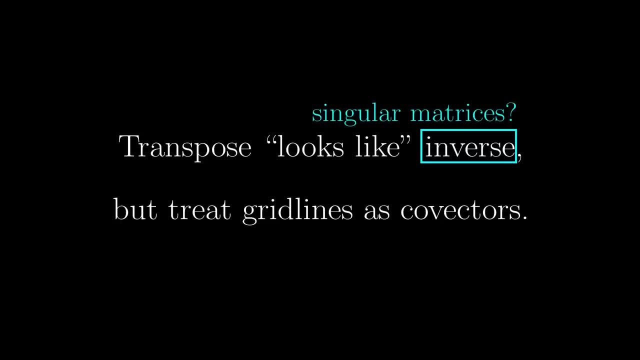 And yes, indeed there is a bit of limitation when it comes to singular matrices and, in general, in technical terms, the rank is smaller than the dimension of your original space. But those are all the cases where the visualization fails. And even in those cases, 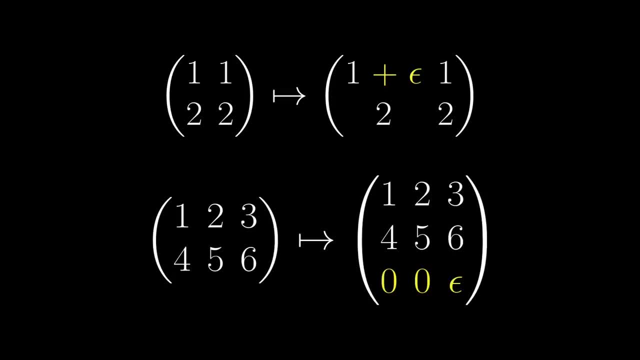 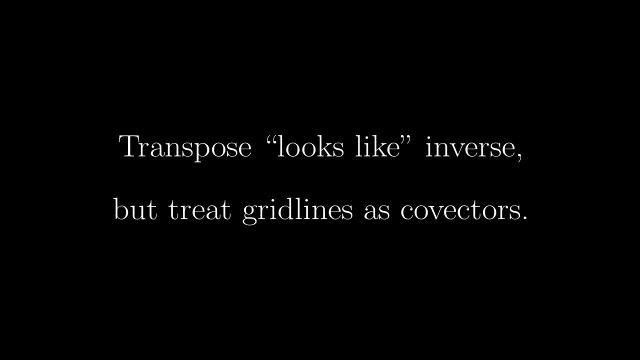 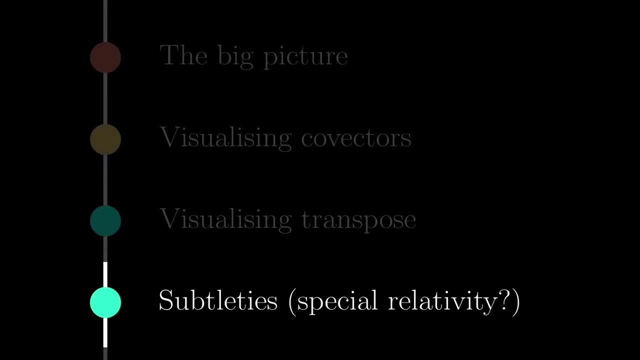 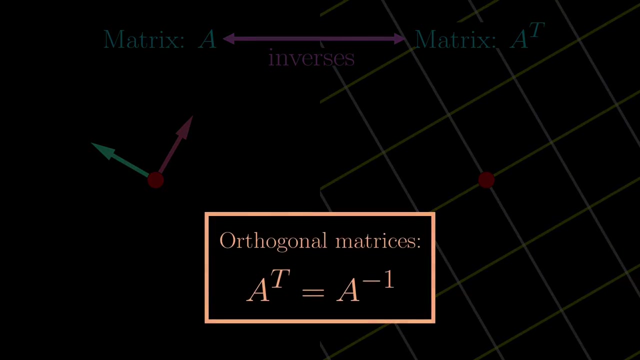 you can still sort of displace your linear maps a tiny little bit to do the visualization. So this really is a powerful visualization for transposes. I want to emphasize a very subtle and technical but important point: The orthogonality condition- A transpose equals A inverse- should not have made any sense to you. 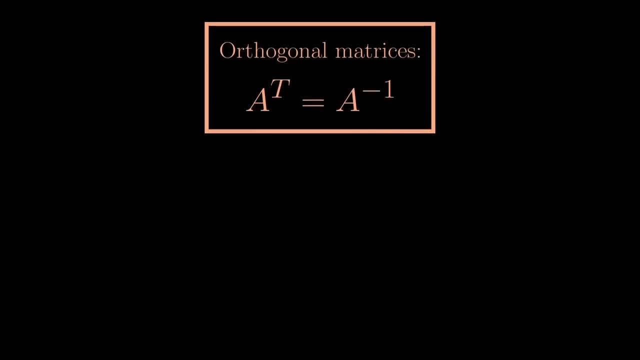 On the left hand side, the transpose is supposed to transform covectors to covectors, But on the right, A inverse transforms vectors to vectors. They aren't even the same type of object. how can they be equal? Well, the trick is to pair up vectors and covectors, treating them sort of the same. 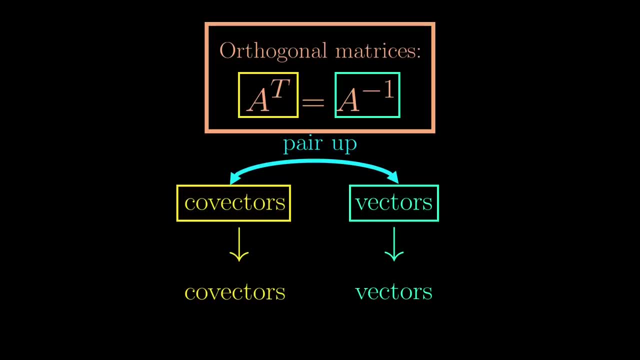 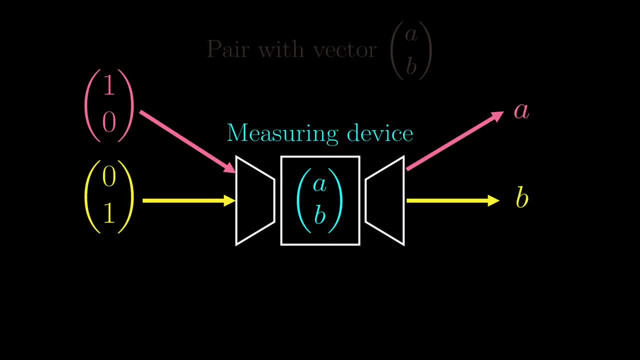 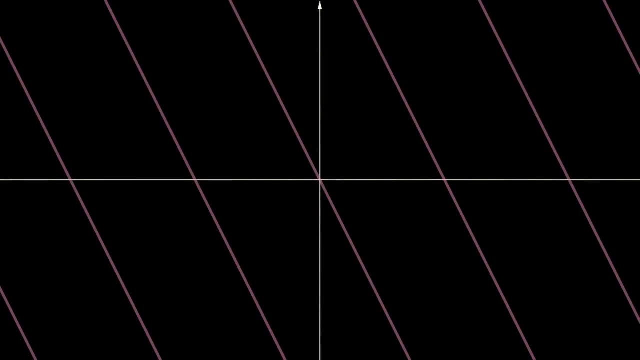 which is what we have done in this video. For this A- B covector, where we measure 1, 0 as A, 0, 1 as B, we have associated with it the vector A- B Or, in the visualization of covectors, as a bunch of parallel lines, we have associated it with. 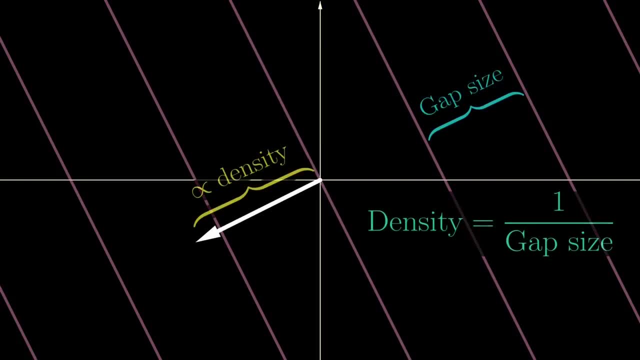 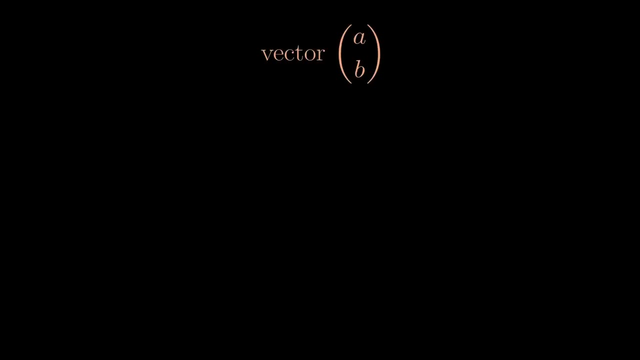 the vector perpendicular to the lines, and length being the density of the lines. Of course we can do the other way around as well. Given the vector, we can draw those parallel lines, and given the vector A- B, we can also easily construct that covector. That's how we have. 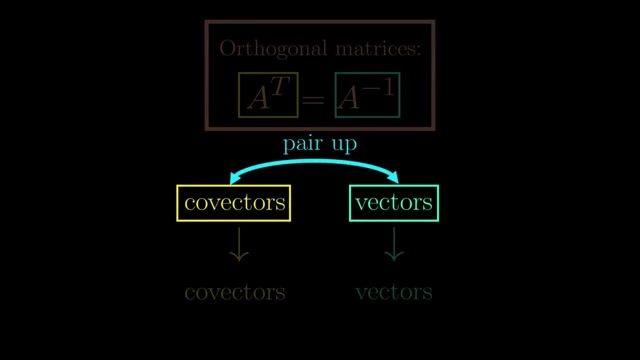 achieved the 1: 0 covector. And that's how we have achieved the 1: 0 covector. This is a very interesting example of a 1 to 1 correspondence between vectors and covectors. A technical remark is that this has to be a linear correspondence, which our pairing is. 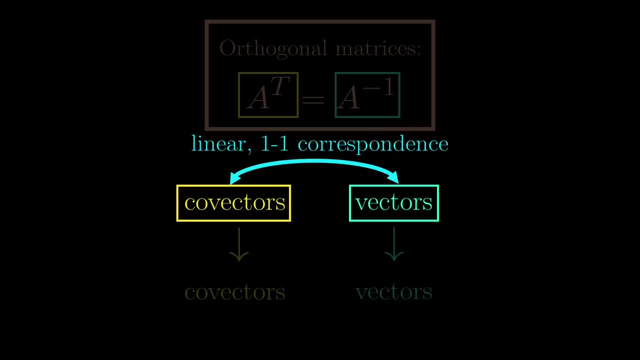 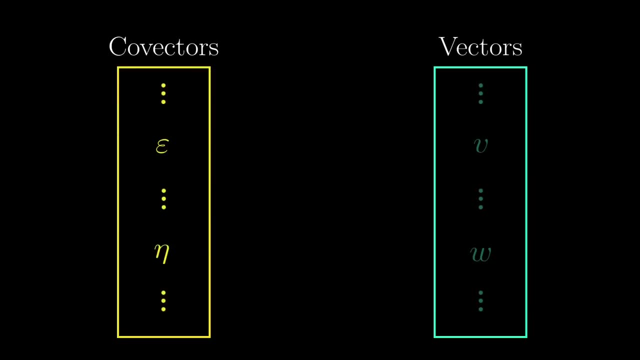 but we don't have to go into the details of what linear means in this context. Let's list a bunch of vectors and covectors that we have. If a transformation transforms a covector epsilon to another covector, eta, an epsilon is paired up. 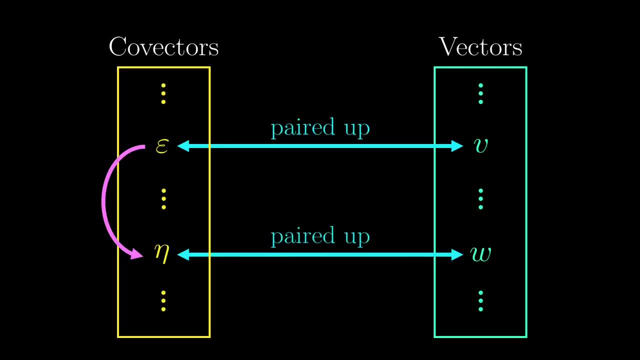 with the vector v, Eta with the vector w, then it looks as if v is being transformed to w. This covector to covector transformation does not even know the existence of v, but because of this pairing we can treat this as a vector to vector transformation. 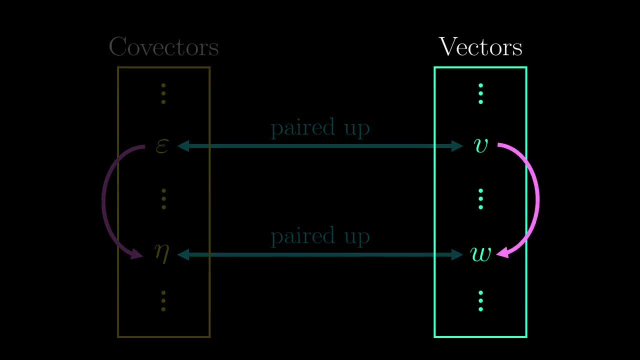 In a similar way, if a vector to vector transformation transforms v to w, we can think of it as two vectors Transforming from epsilon to eta. It is in this sense that we say something like A transpose equals A inverse. There are two reasons why I want to emphasise the process of pairing up. First, 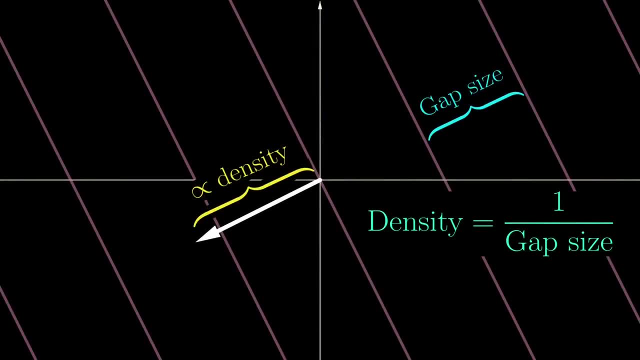 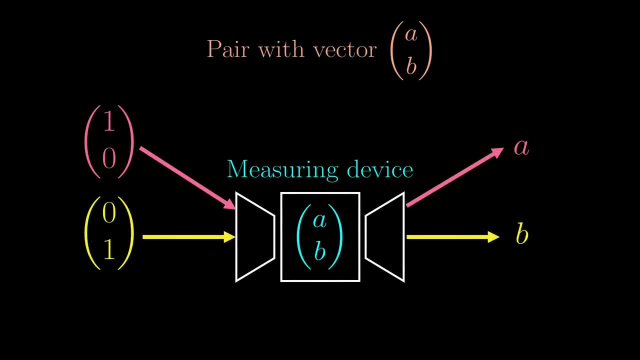 while this way of identifying a vector with a covector is very standard and very natural, this is not the only way of doing it. You could have also paired up with the vector negative A B instead or A negative B. These will still yield a 1 to 1 correspondence. There are many 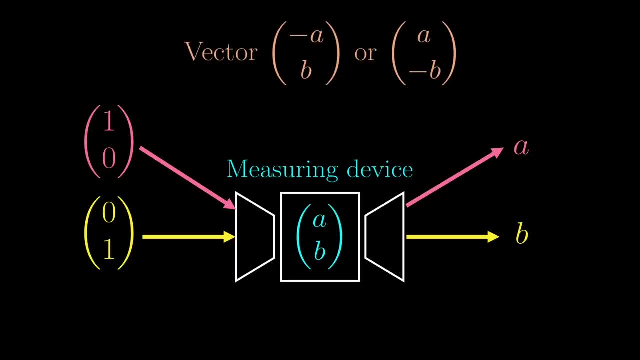 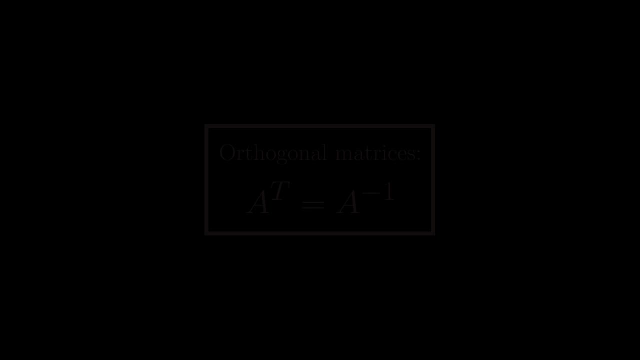 other options, but I'm choosing these two simply because either of these two will give you the mathematics of special relativity in 1 plus 1 dimensions and any matrix that fulfils this orthogonality condition under this pairing are the Lorenz transformations. Don't worry if any of 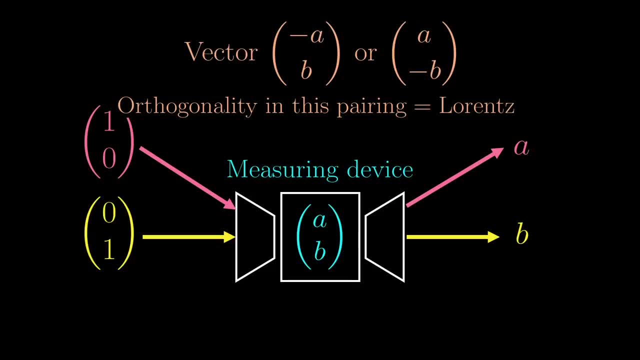 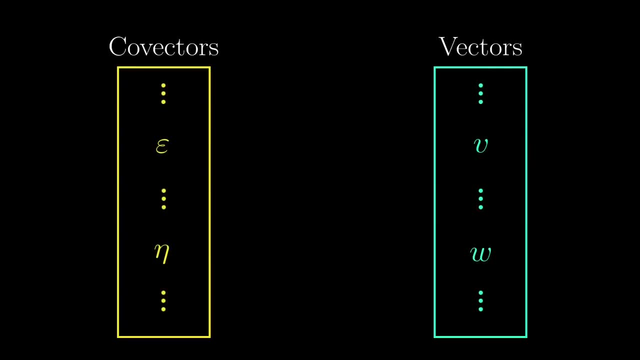 these doesn't make sense. I will probably make videos on special and general relativity later on. If you know something about relativity and are wondering why this has anything to do with it, know that the act of going from vectors to covectors is the job of the metric tensor. 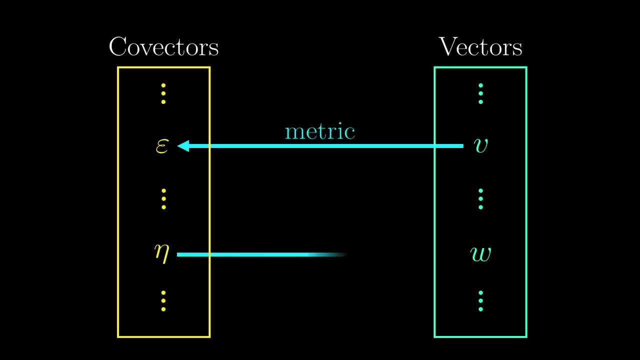 or metric for short, And going from covectors to vectors is the job of the inverse metric. Anyway, the point is, it is very important to specify which 1 to 1 correspondence or the metric you are using, because different metrics yield different mathematics. The other thing is that you might not even be able to pair those up. 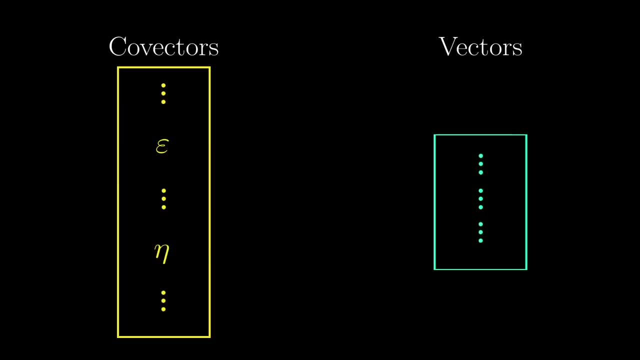 In infinite dimensional vector spaces there are way more covectors than vectors, so you can never achieve a 1 to 1 correspondence. If you still insist on trying to define orthogonality, then you need to restrict the kind of covectors you consider. 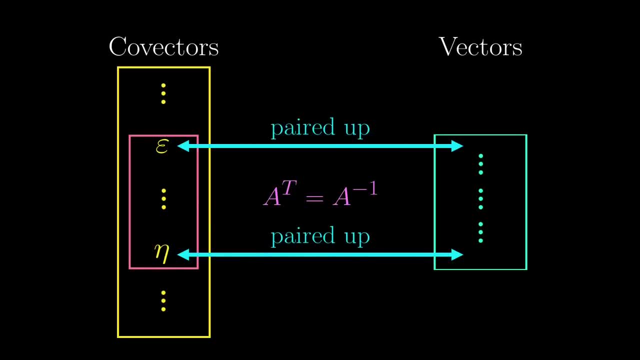 and hope that those special covectors have a 1 to 1 correspondence with the vectors. This will be better explained with the concept of an adjoint which I have put some resources in the description. This adjoint concept is the bread and butter of quantum mechanics. 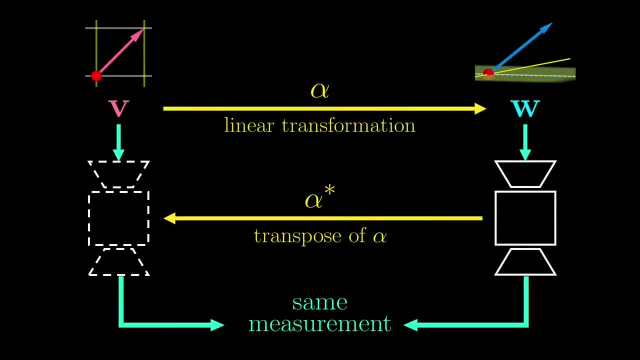 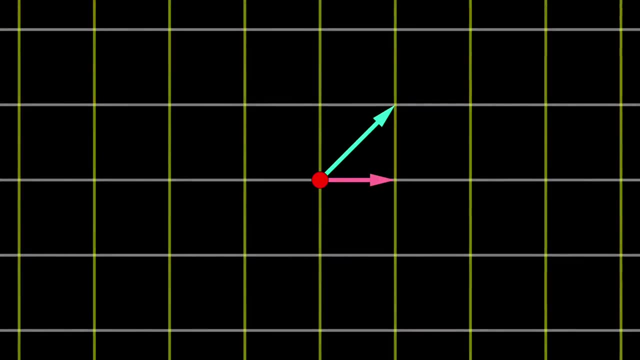 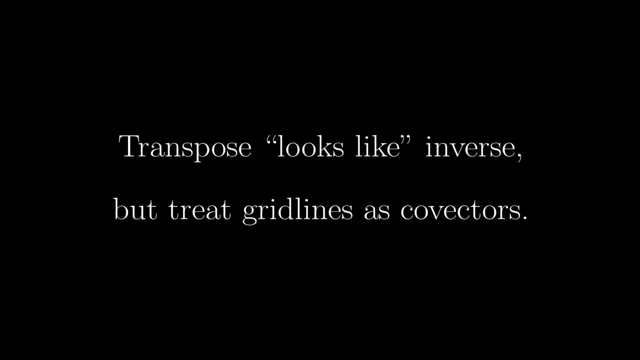 So in this video we have the big picture of the transpose and used it to visually visualize transpose with a few examples like shear, as you see here, as well as diagonal matrices and rotations, deducing that transposes do look like inverses. but we have to treat those. 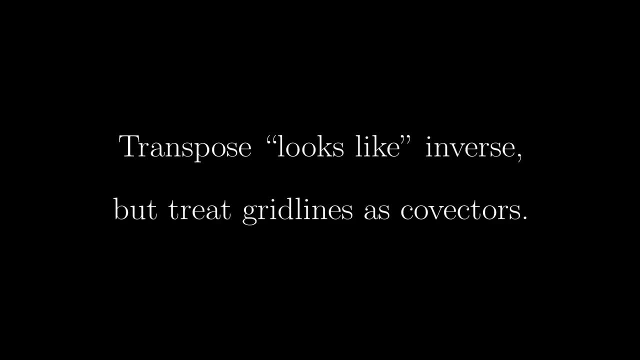 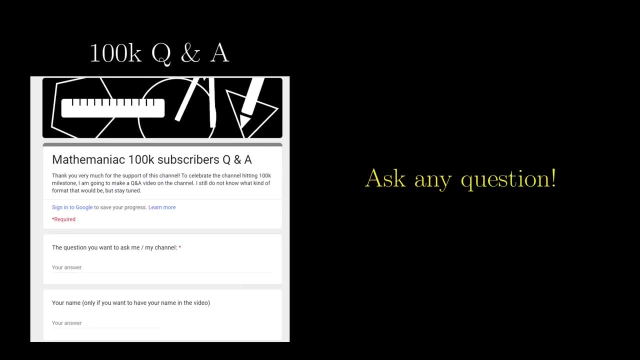 grid lines as covectors. By the way, I'm still collecting questions for the 100,000 subscribers Q&A. so if you want to ask any questions, this is the last chance to ask because if everything goes well, next video will be it. But please do not ask any animation-related questions anymore.